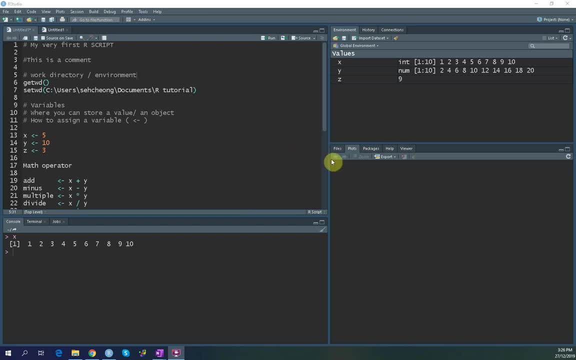 Hi, welcome to this number three tutorial of this series, and in this video I'm going to teach, teach you about R basic syntax and yeah, so let's get started. so the very first thing I will talk about is a command. so when you are writing an R script is you will probably put in some notes that you 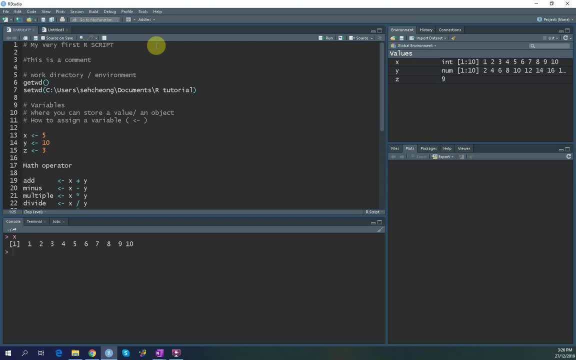 want to let maybe yourself in the future to understand what you were writing, and also to someone who were reading your script to understand what you are trying to do with this command. so then, in R, the way we put a command is by using the hashtag key, as you can see here. so by adding a. 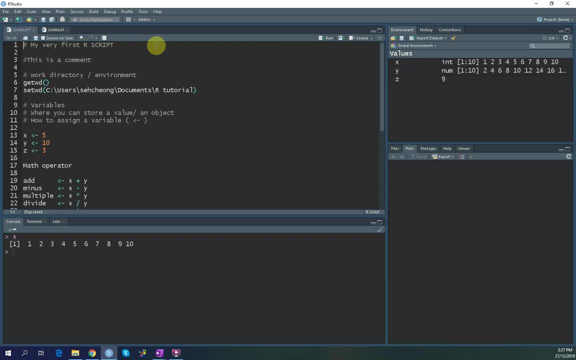 hashtag at the beginning of the line. I can change line number one into a command. you can see here the color turns gray and it means that is now a command, which means when you run the script, R will ignore this line and it will not be run as a code. all right, so yeah, you can see, here is the same. so 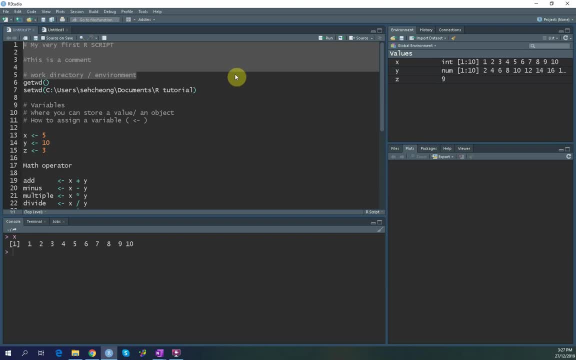 let's say, if I want to command several lines, I can simply just select all of them and just press ctrl shift C so you can see up. sorry, I should try with these two lines. all right, ctrl shift C, it will turn these two lines into command by doing the same thing. if you uncomment that, two lines, all right. 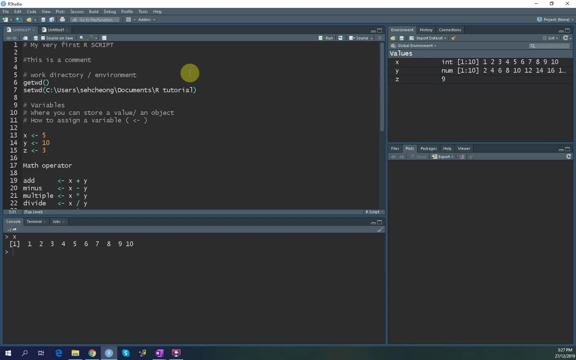 so this is how we use the command in our script. so the next one is to understand the work directory or environment that we are currently in. so you like, even though you are writing a R script, you like when you are writing using a word document. when you are writing, you need to know where these 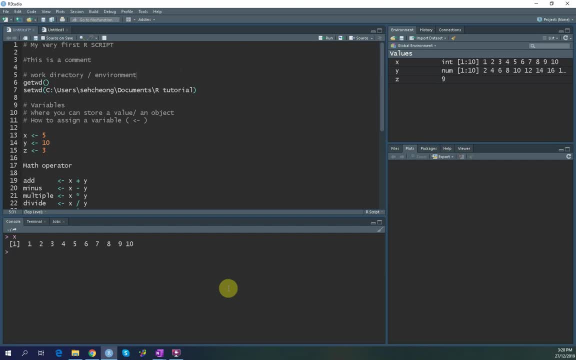 documents are safe or where which, in which folder I'm currently currently working on. so the way to know, the current directory is running a command called getwd. so here, so I've already typed get wd. so it means that work directory. and don't forget the payment code, because our current 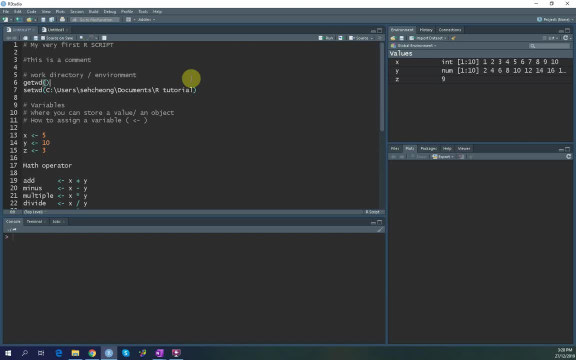 and don't forget the parenthesis after that. so if you want to run this line, you can simply select this line, use run, press the run button or you can over here and you can see the result over here. so I'm currently on my C Drive, users folder Sejong, my folder and documents folder. all right, or you can. 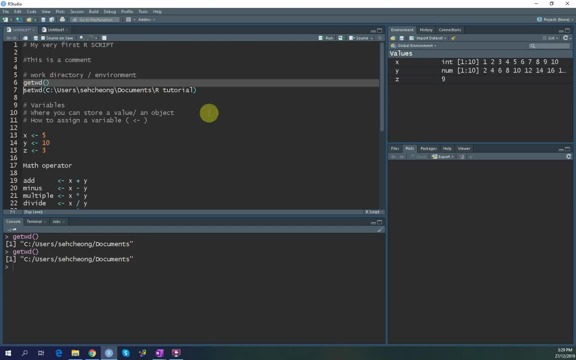 just select this line and press ctrl enter and you will get the same results. okay, okay, let's say, if you want to change, this is not them the working directory that you want, you can use this function, setwd, which is set works directory directory, to change it to the folder that you want. so let's say, if, let 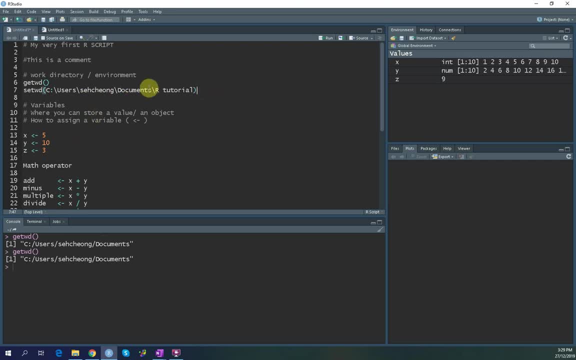 let's try this command. okay. so if let's say I've created one folder in the documents folder which call our tutorial, and let's say, if you want, if I run this, come on. so by putting the cursor in line number seven and press ctrl enter, it means it will run the command on that line. okay. 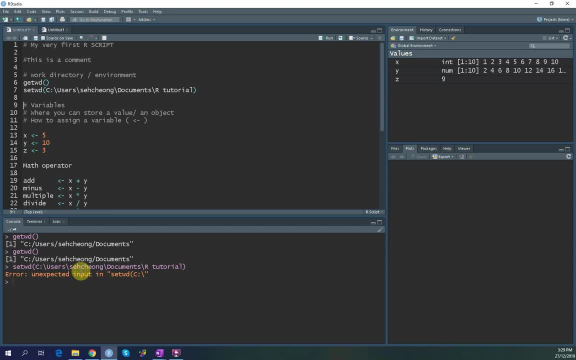 so and see, so there's an error over there. so let's see what's wrong with the error. okay, so I think I found one. so let's see. okay, in this one you should put the path of the folder in the quote, all right, so let's try it again. and then, if something's wrong. so the reason is that. 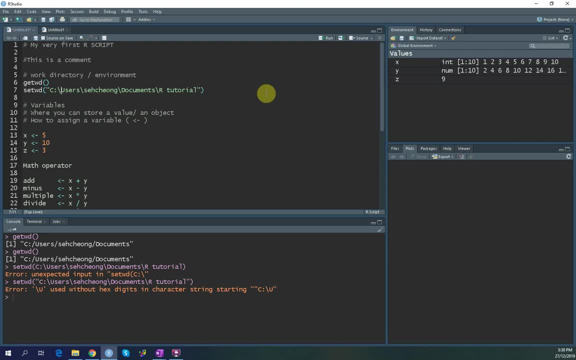 because of the back. backslash is kind of like the special characters in in our programming. so if you want to on want to tell our backslash is something that you need, you need to use another backslash to tell our we escape the backslash. so So let me try all this, putting another backslash in front of it, and I try- oh sorry, ctrl enter. 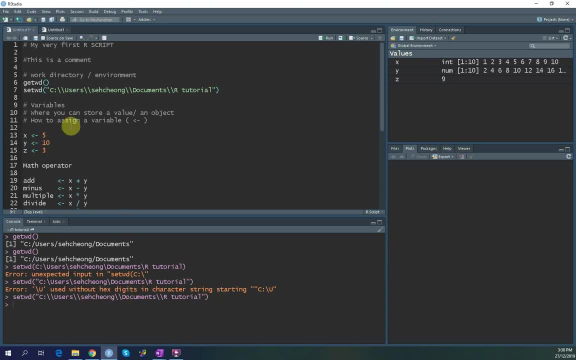 So this time we don't have any error. So let's use getwd again to check which working directory we are currently on. So run it again So you can see here. now I successfully changed the working directory into our tutorial folder. So let's say, if I want to save my current script, okay, save. 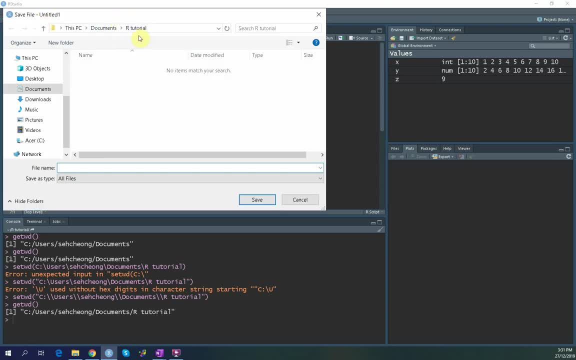 So I'm in our tutorial. If you want to find a path- if you don't know which the path of that, you can open a file explorer and click on this. Then you can see the path. So you'll be over there, over here. 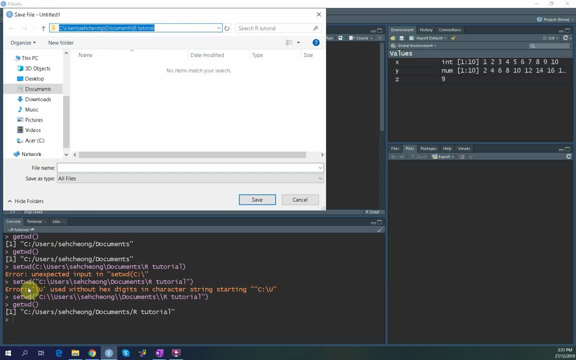 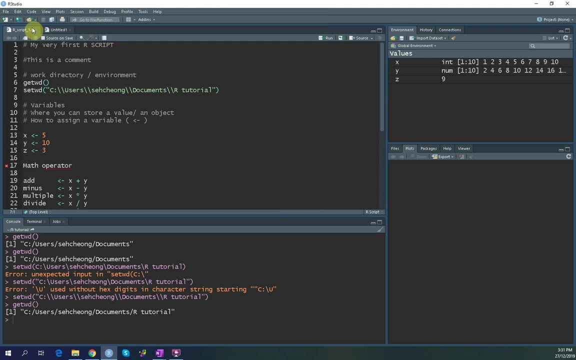 So you can just copy it and paste into this setwd function so that you can change it. So let's say I save this one is our script number one, and just simply save that And you can see here: it's saved in the r format. 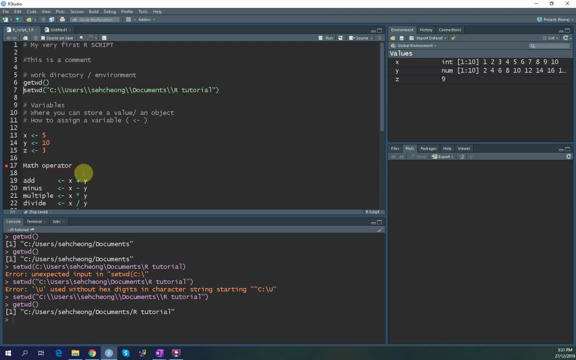 So this is our script format, Okay, Okay. So when I save something And r will automatically detect this, Detect every line in this script, whether it's a valid command or not. Over here you can see these are some commands that I forgot to put hashtag on it. 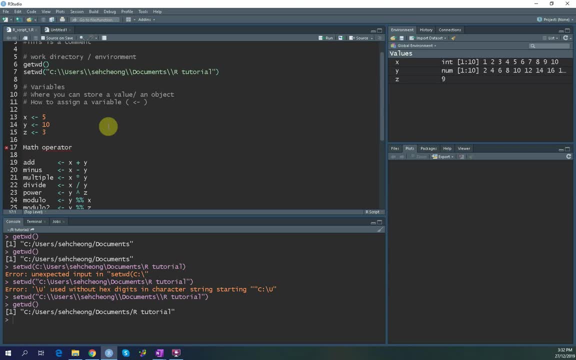 And you will see there's an error over there. So let's see if I could hashtag: over here, over here, Let's see this one over here, Yep, And then you won't have any error. Okay, So after this book directory and we will move on to the next thing, which is the variables. 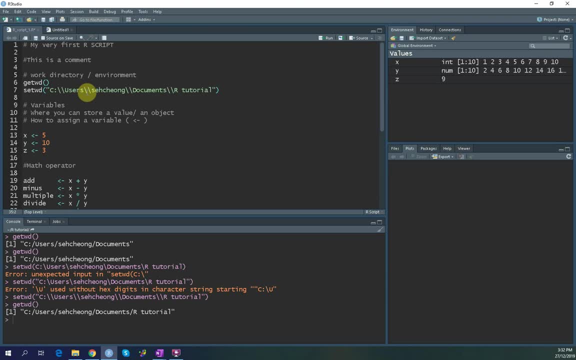 So variables is a very important concept in, I think, any programming language, So in r. variable is something where you can store a value or an object, And And how to assign a variable is by using this. It's a symbol. 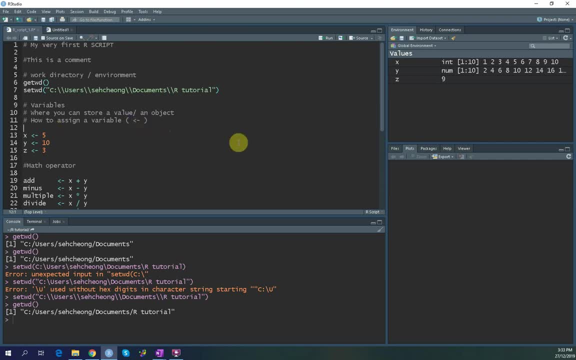 It's smaller than and minus. So, yeah, you might find it a bit weird at the beginning. It's like you want to type it every time. It's not that intuitive, But there's a shortcut key that you can use. It's alternate. 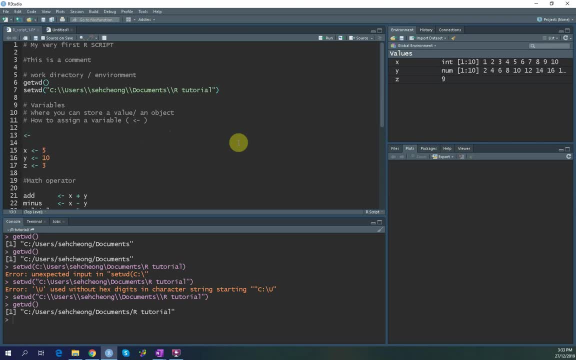 So it's alternate plus, minus. So if I hold alternate and minus, it will automatically give an assigned symbol. Okay, So if I hold alternate and minus, it will automatically give an assigned symbol. Okay, So, Okay. So assign a variable in r is very simple. 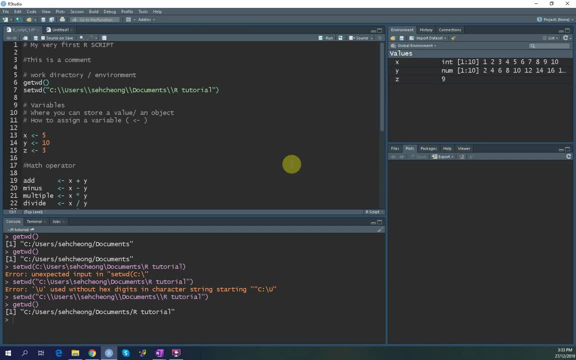 So you just simply put the name of the variable. So in this line, number 3, 13,, I put x, I assign 5 as a value to x, Yep And 10 to y. So y as a variable name. 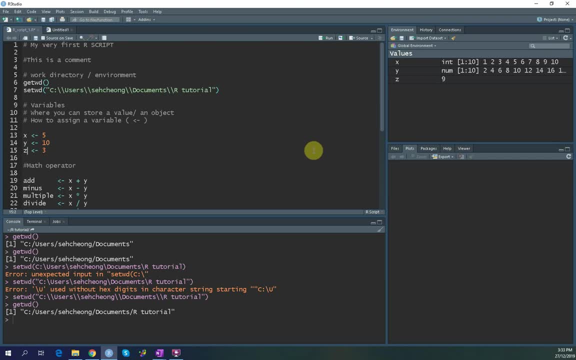 And 3 as the value of z variable. So in r, if you want to call a variable, we'll just simply Type the name of the variable. Let's say: I want to know what's. So. first of all you need to run this line. 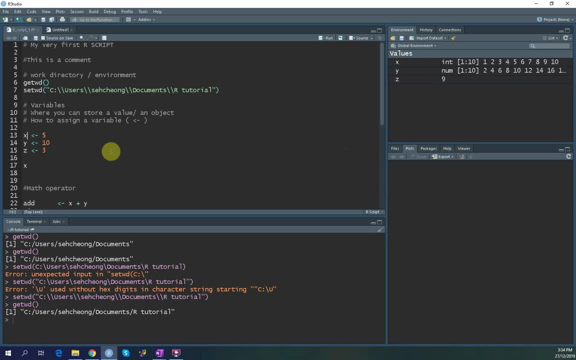 Because, let's say previously, I've created a variable, x, And these are the value of this variable. You can see, it's not only one value. Actually, a variable can contain up to thousands of value. It depends on what you want to call it. 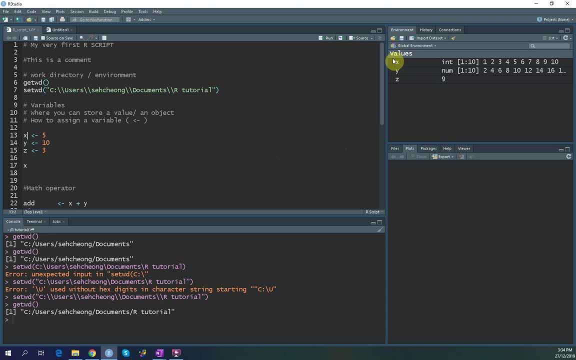 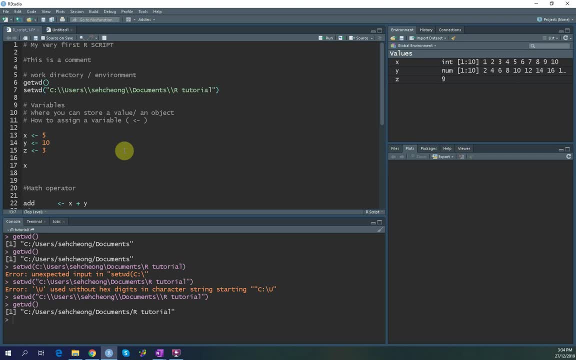 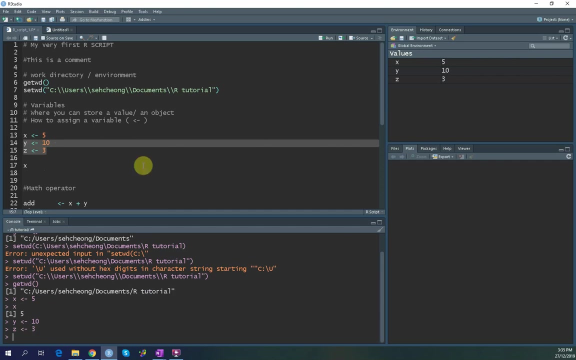 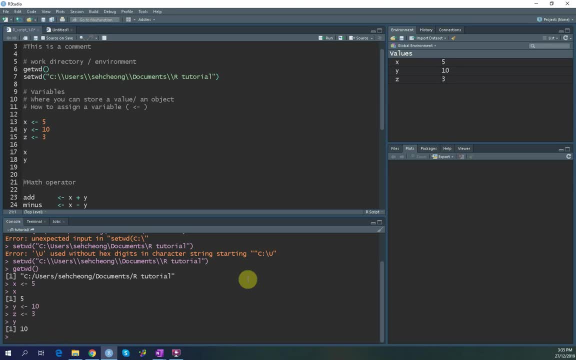 right here, or you can come to the console, just type y, enter, and you will get the value in y. so so when I assign- so just now- X was a list of values. so then when I reassign X again, it will replace all the values of the previous. 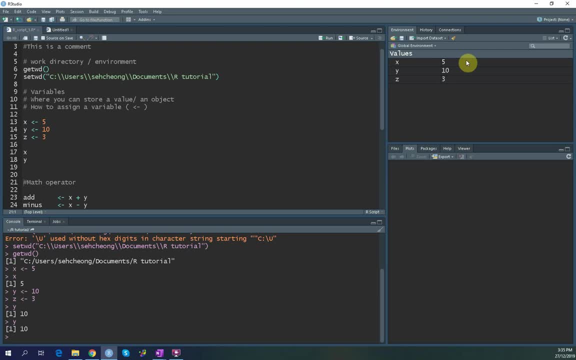 variables. having the, that is having the same name. so be aware of this, so you don't want to lose your variable. so you might want to give a better or a more easy to understand variable name so that you don't mess up with the old variable, that you still need it. and one thing is that 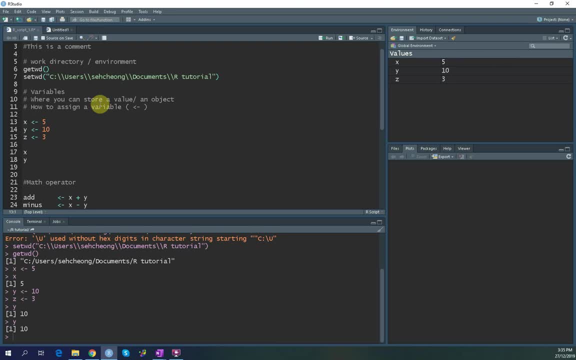 you still need it. and one thing is that you still need it, and one thing is that a variable doesn't start with a number. a variable doesn't start with a number. a variable doesn't start with a number. you can't assign a variable with starting. you can't assign a variable with starting. 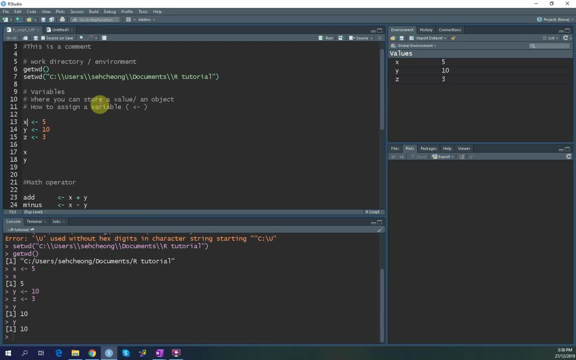 you can't assign a variable with starting with a number or any special symbol. the with a number or any special symbol. the with a number or any special symbol. the best thing is to start with a letter and best thing is to start with a letter and best thing is to start with a letter, and and the variable can accept underscore.